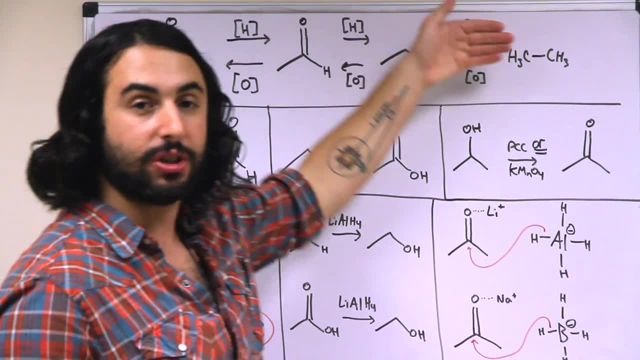 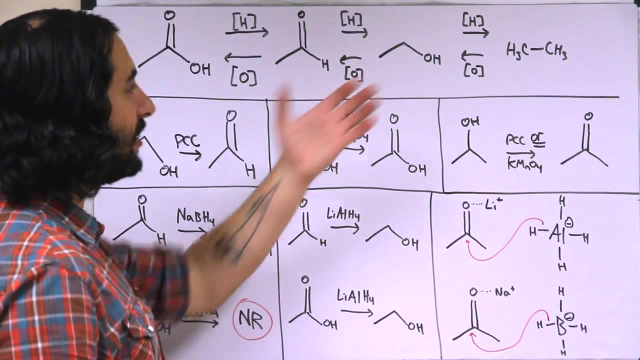 So let's go ahead and get started. Let's get started, All right, so we've got a new little. this direction, this is reduction. in this direction, this is oxidation. so there are different compounds that will induce different transformations, so there are reducing agents that will reduce any of 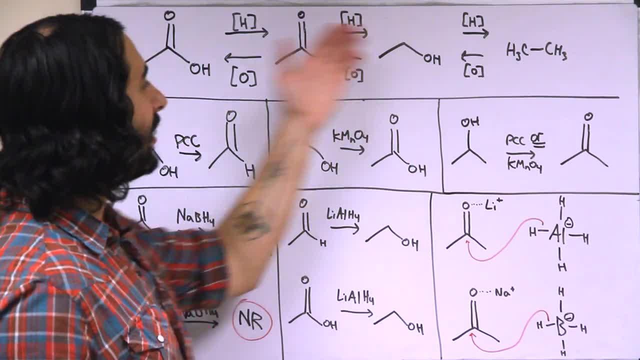 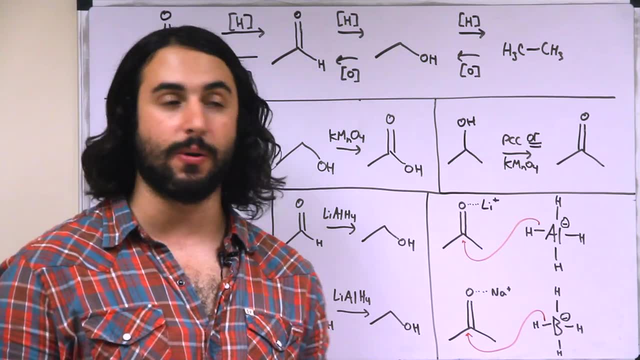 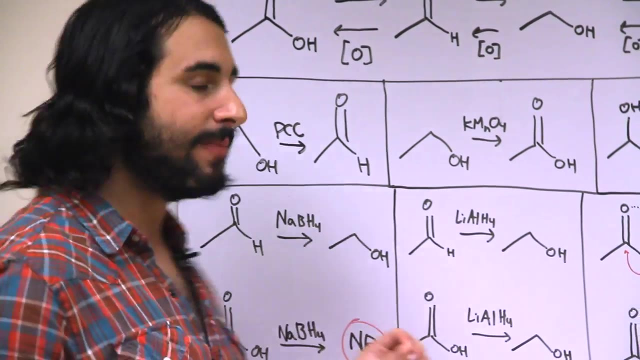 these compounds in this direction and there are oxidizing agents that will oxidize compounds into this direction. so let's take a look at a few of them and see how they differ in strength and why we might use one over another. so just to take a look at oxidations: we can oxidize primary or secondary. alcohols. so a tertiary alcohol cannot be oxidized because that carbon already has three bonds to other carbons. so there are not any bonds that can be replaced to give that carbon more bonds to oxygen. we can only lose bonds to hydrogen. so 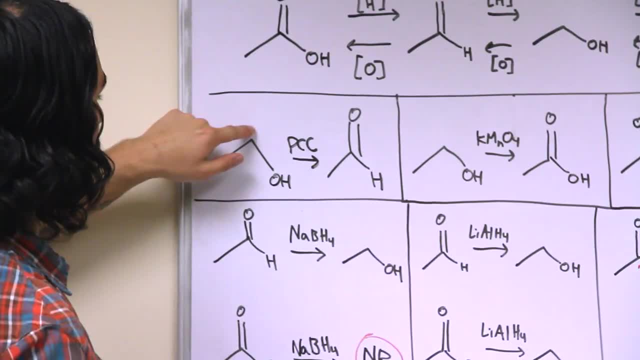 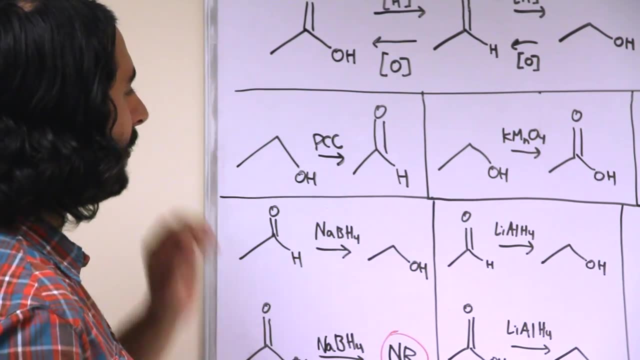 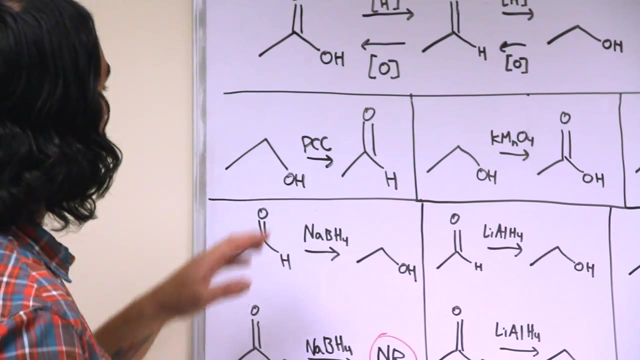 this carbon here has one bond to oxygen and has two bonds to hydrogen, so it is going to be possible to gain more oxygen content here. now a primary alcohol can be oxidized either to the aldehyde or to the carboxylic acid level of functional group, so PCC. 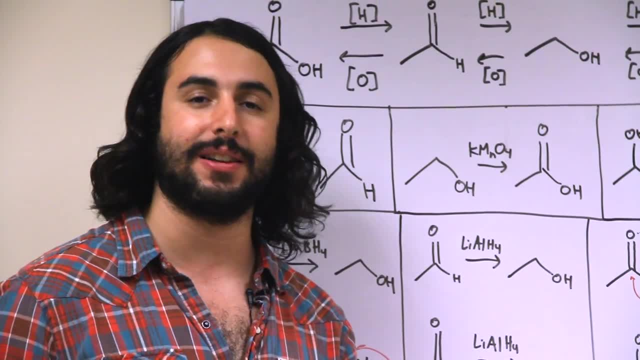 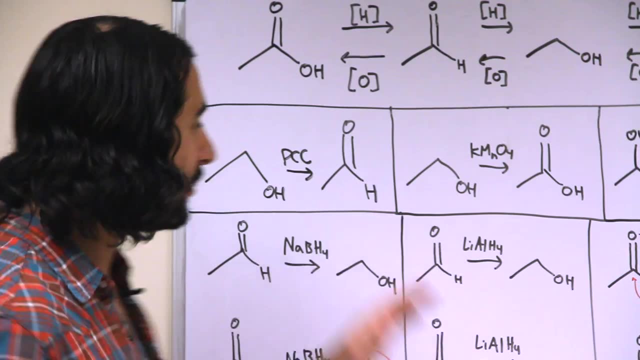 pyridinium chlorochromate. this is a softer oxidizing agent that is only going to oxidize primary alcohol to the aldehyde functional group level, so it's going to stop there with two bonds to oxygen, something stronger like potassium permanganate or chromic acid or something else. is going to take a primary alcohol and oxidize all the way to the carboxylic acid functional group level. so, depending on what you're going for in, say, a synthetic pathway or something that might guide you in terms of what oxidizing agent you want to use, now, a secondary alcohol can only. 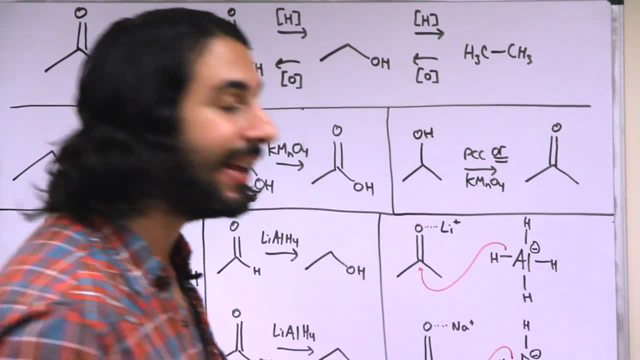 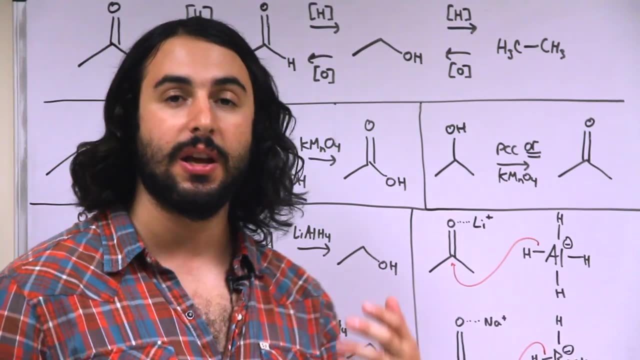 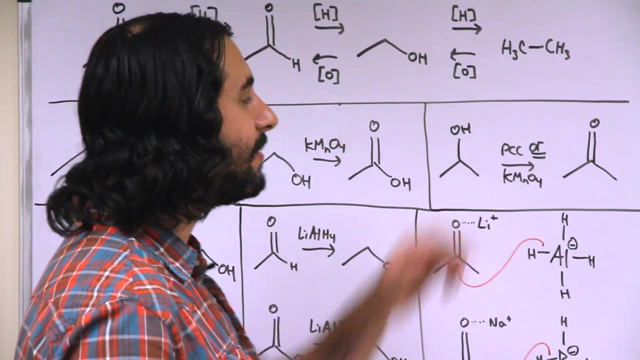 be oxidized to the ketone functional group level. because we can oxidize any further. there's only one additional bond to hydrogen that can be. that can be replaced with another bond to oxygen. we're not going to break any of these carbon-carbon bonds, so for a secondary alcohol it doesn't matter. 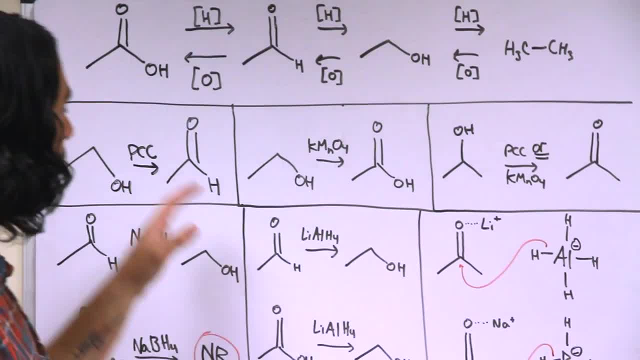 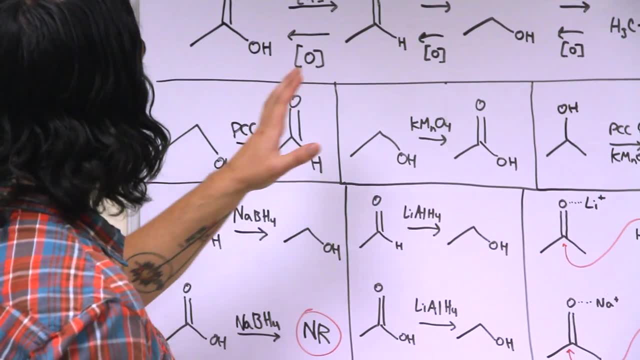 which we're going to use. we're just going to get a ketone, so it's mainly for these primary alcohols where we're gonna have to make a decision. so now let's look at reducing agents, whereas oxidizing agents are going to help us go. 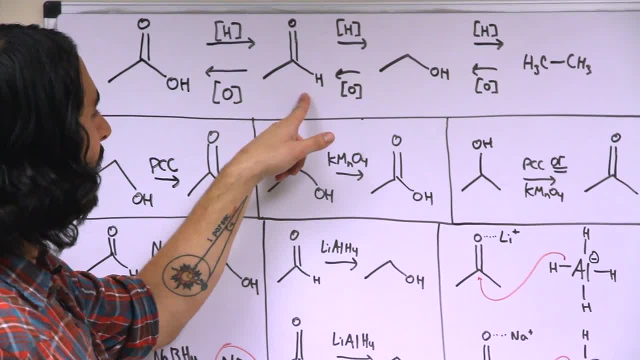 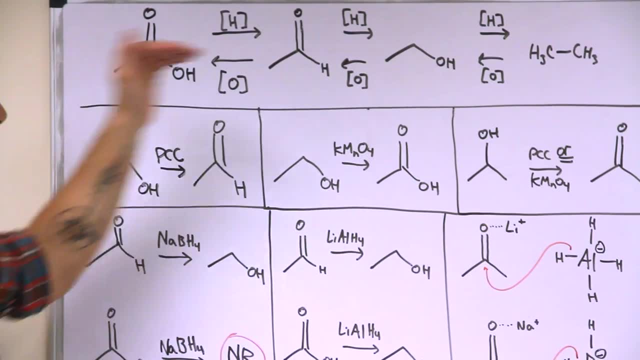 in this direction. we saw that we could go from primary alcohol to aldehyde with the PCC, or primary alcohol directly to carboxylic acid with potassium permanganate. now let's see what's going on in the opposite direction. so we have different reducing agents and again these can have different strengths. so 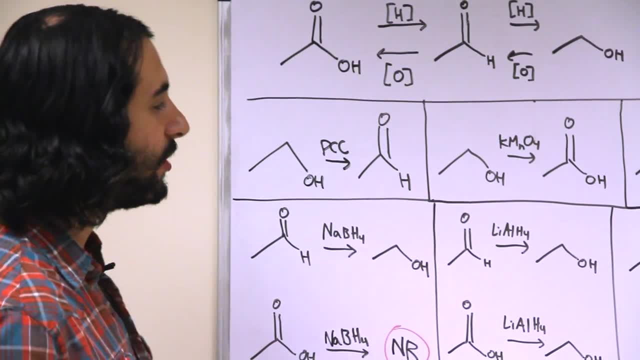 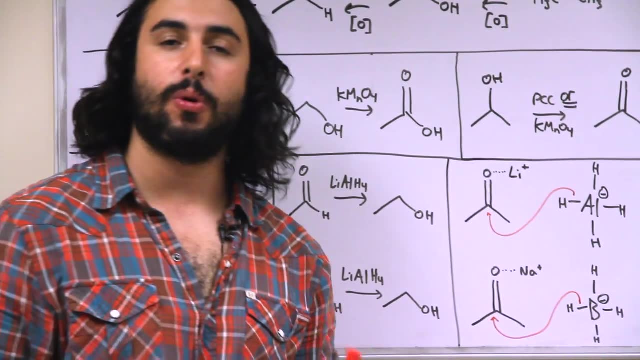 let's take a look at something like sodium borohydride. that's NABH4. so we have borohydride with a sodium counter ion. so this is BH4-. now boron has three valence electrons, so it's going to have a tendency to make three covalent. 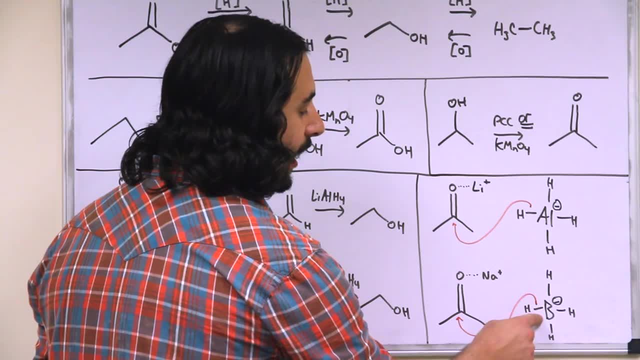 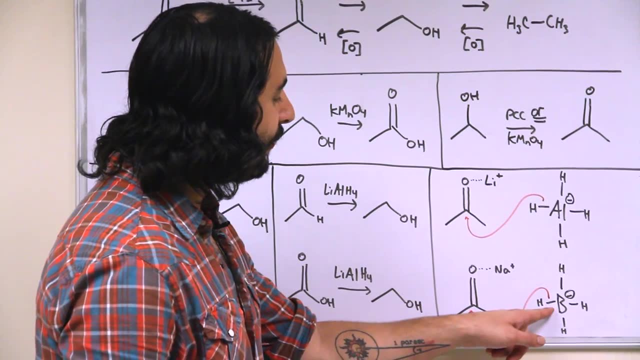 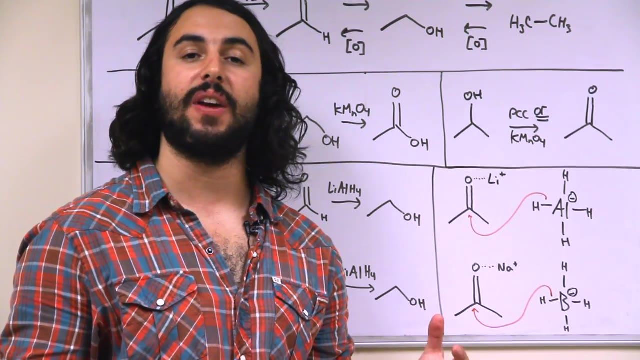 bonds. but now that it has a fourth here, this, the boron is going to have a formal negative charge. so it is going to be very interested in losing a hydride. so if H- leaves, leaving just BH3, that boron is going to neutralize and that's an energetically favorable situation. so 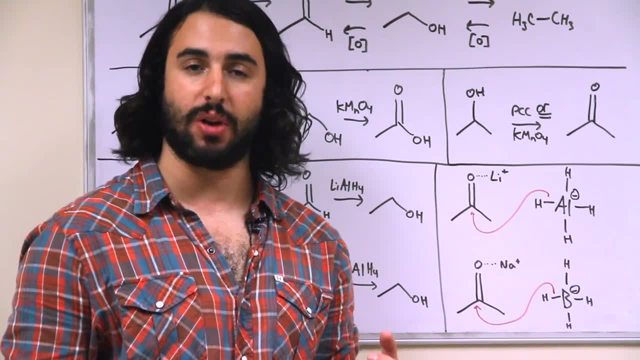 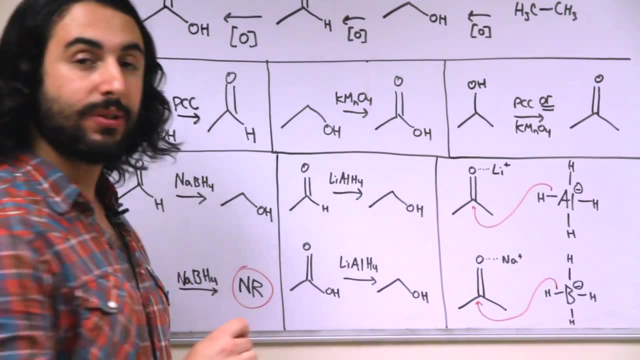 that's why sodium borohydride is a good source of hydride or an H- nucleophile, so hydrides have a tendency to attack carbonyls, thus reducing them. so what we're looking at here is sodium borohydride is capable of reducing an. 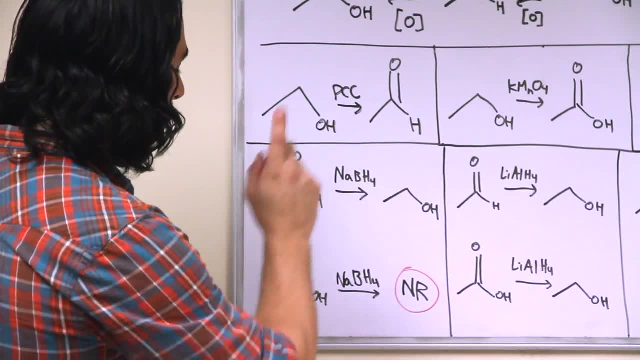 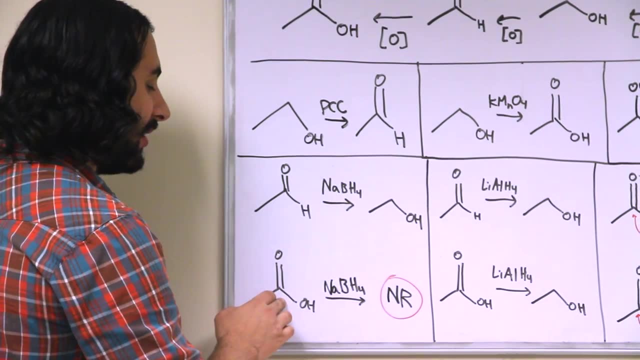 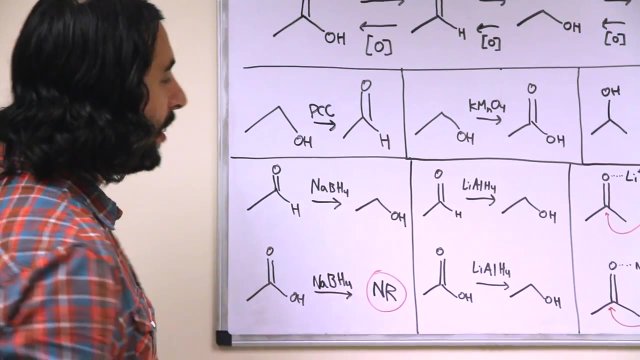 aldehyde to the alcohol functional group level. however it is, it is a. it is a soft reducing agent. it does not have the strength to reduce something like a carboxylic acid. so in the presence of NABH4 there will be no reaction with it, with a carboxylic acid. but there are. 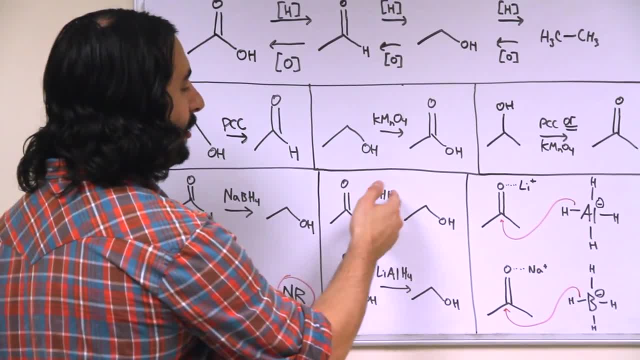 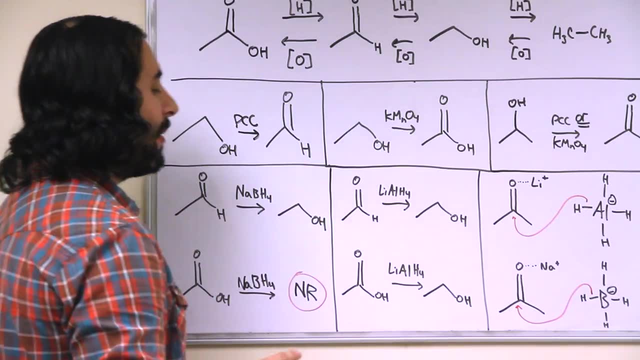 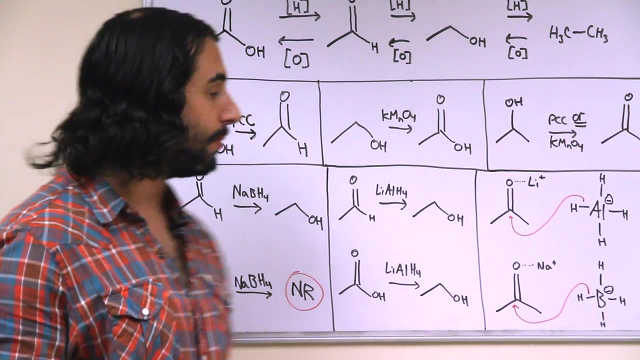 stronger or harder reducing agents like, say, lithium aluminum hydride. so here is an aldehyde that can be reduced perfectly well with lithium aluminum hydride, but lithium aluminum hydride is also strong enough to reduce the carboxylic acid all the way to the primary alcohol functional group level. so let's take a. 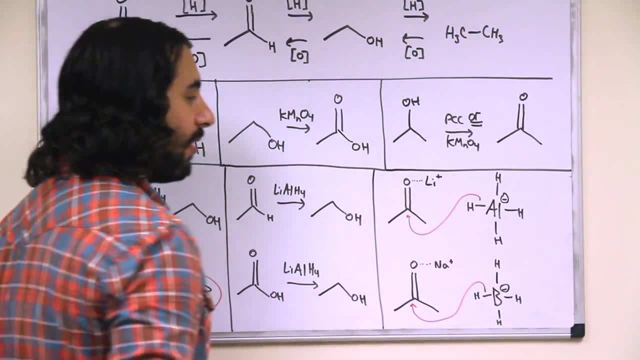 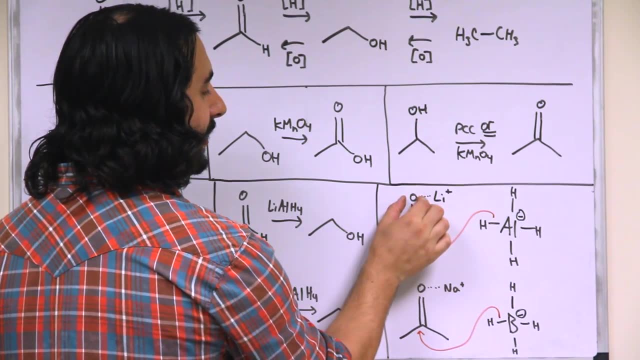 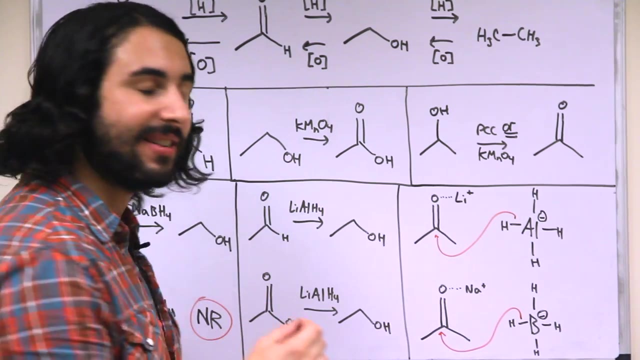 look at why that might be so. here's lithium aluminum hydride, here's sodium borohydride. so what happens is that the positively charged counter ion in solution is going to go and coordinate to the oxygen in the carbonyl. now, lithium is a smaller ion, so it's a better lewis acid, so it is going to more. 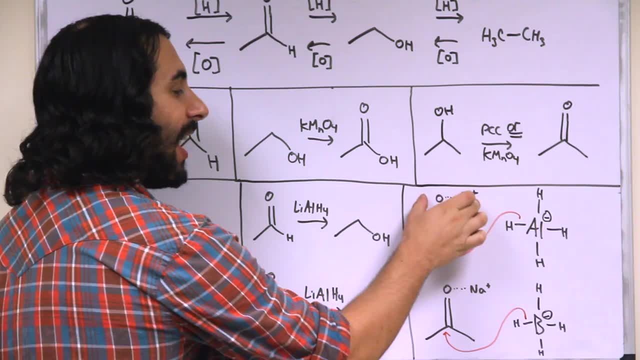 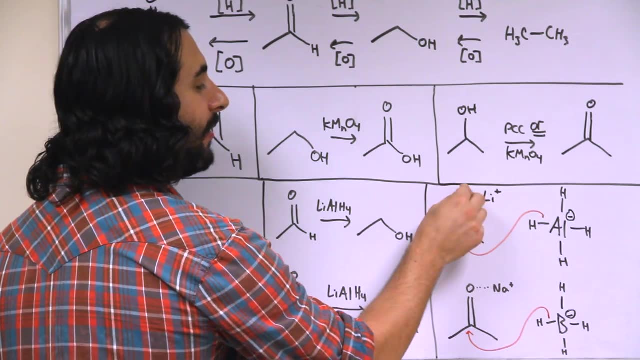 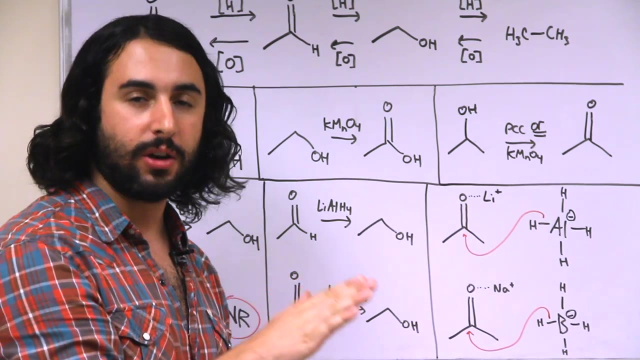 strongly interact in ion-dipole fashion with this oxygen atom. so that is going to generate something of a partial positivity on that oxygen because some of the electron density in the lone pairs is going to be tied up with this partial- it's actually quite strong interaction. it is nearing the level of a.